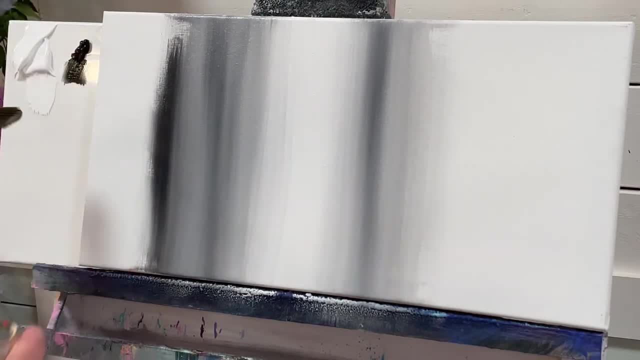 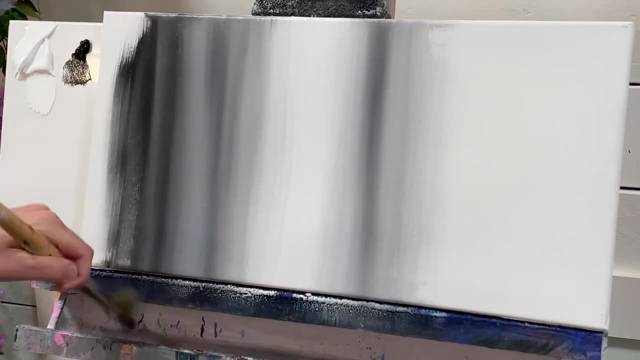 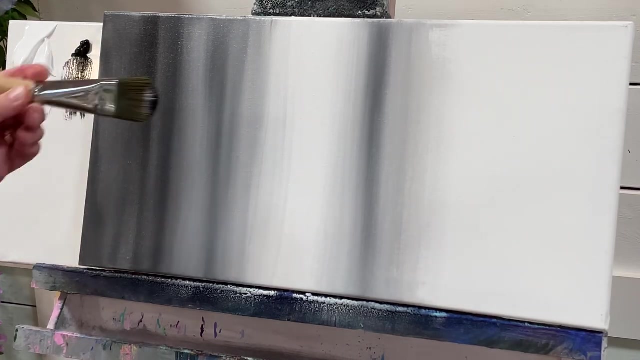 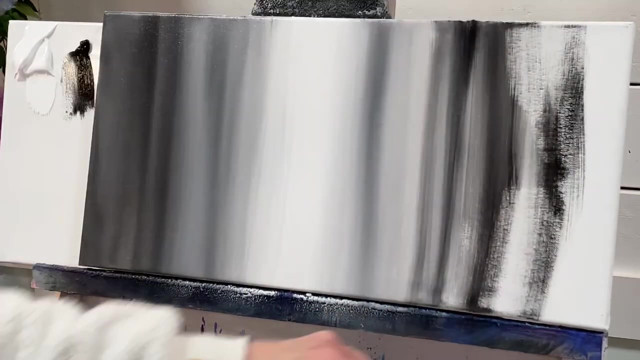 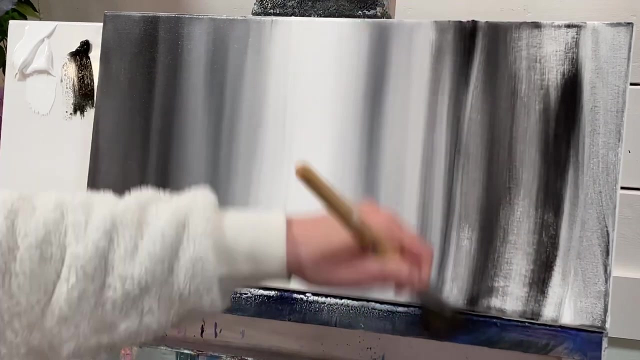 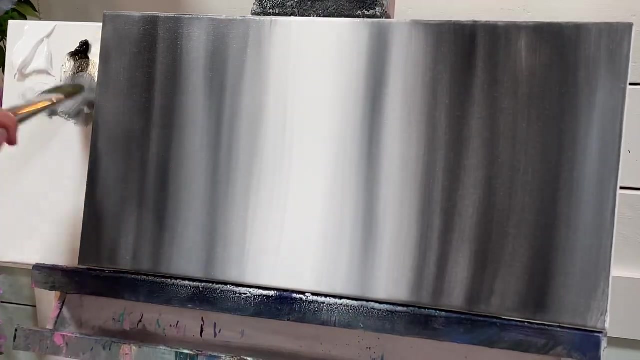 If you need to add a little bit of water, just add the smallest amount. Okay, now I'm going to start on this side doing the same thing. Okay, and you can see, the first one I did has a lot of water in it, so it didn't get helping. 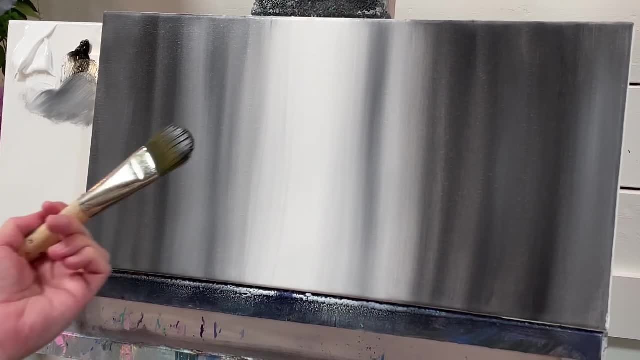 Now the next thing. what I'm going to do is just come right across with the leftover paint. I've hardly got any paint in my brush here. I'm going to go up from the bottom of my canvas 1 inch and I'm going to just 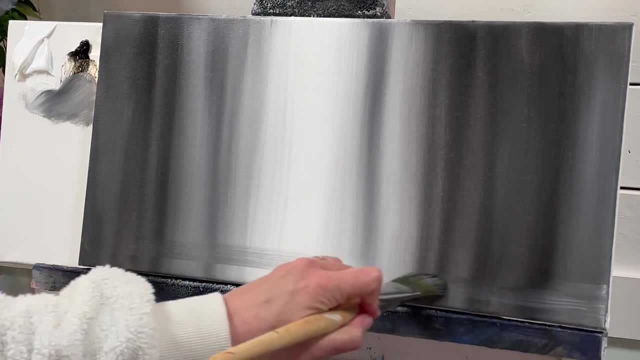 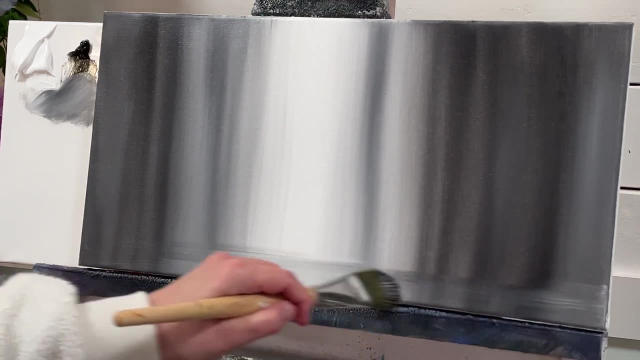 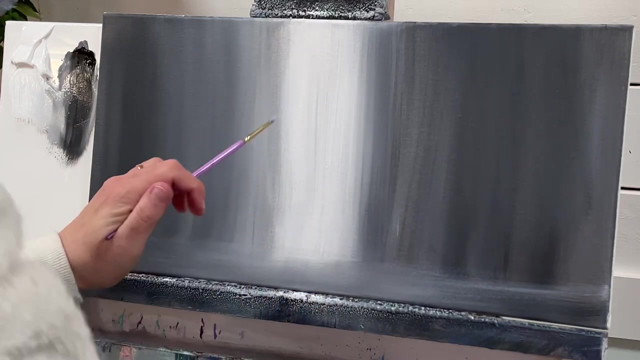 pull off the paint And you can notice. you can see the plaque. paint is moisturizing down the canvas and now we have. okay, now this is all dry, I'm going to use my round brush- it's a number three round brush- and I'm going to start coming in with the figure. I'm going to start with a little bit. 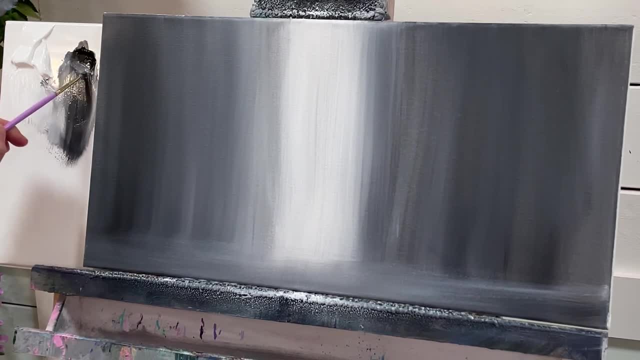 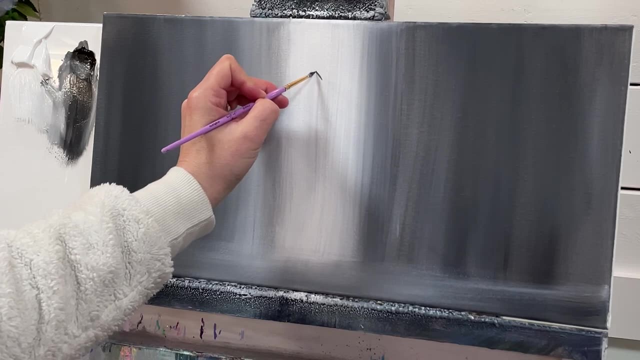 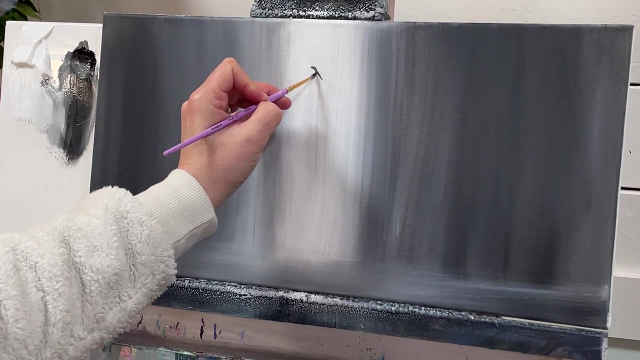 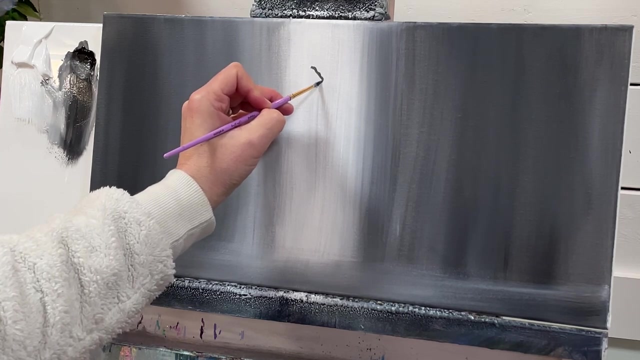 of black, a little bit of white, we'll make a dark gray. and we're going to start with the head right about here. now her, her face is going to be on an angle, so we're going to just kind of come from the forehead up here, in for her eye, slightly out for the nose, and then the mouth and then the. 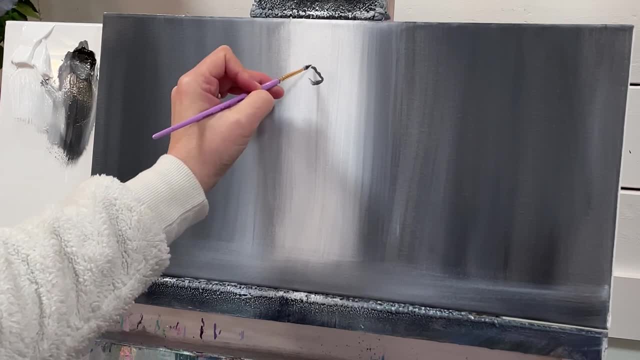 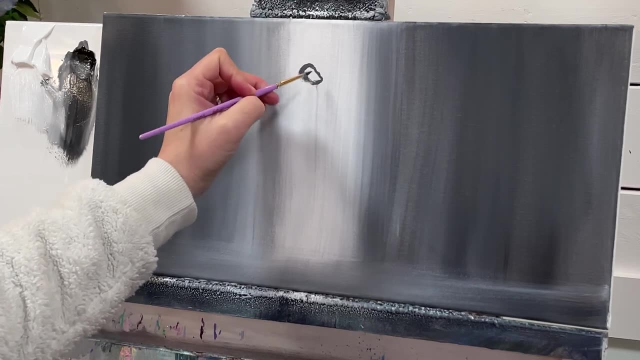 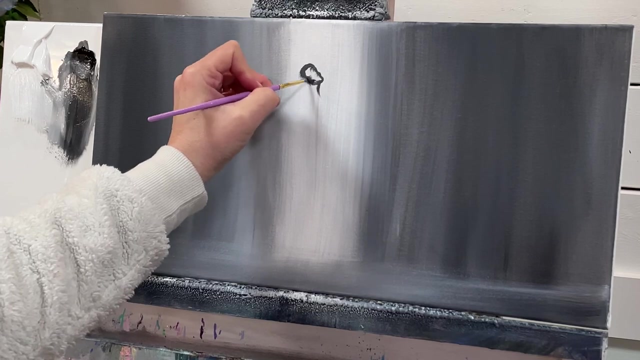 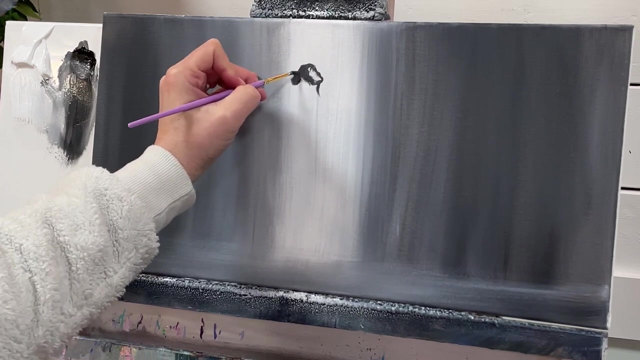 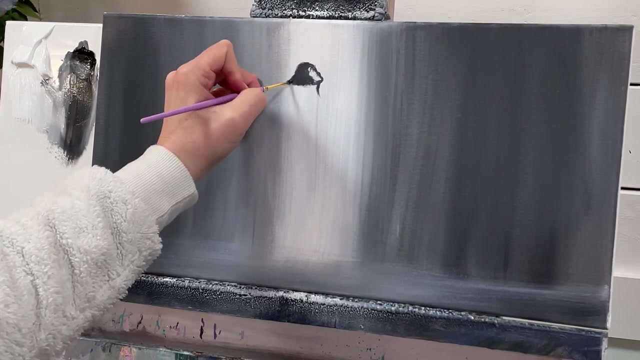 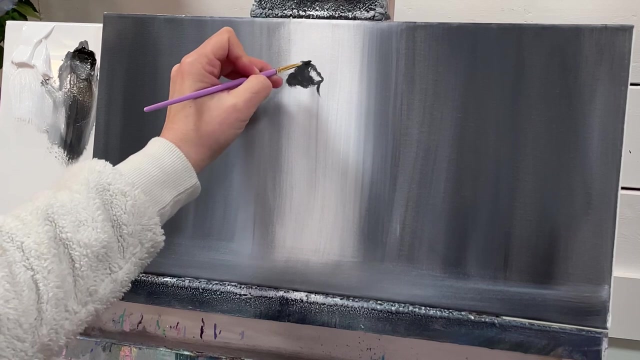 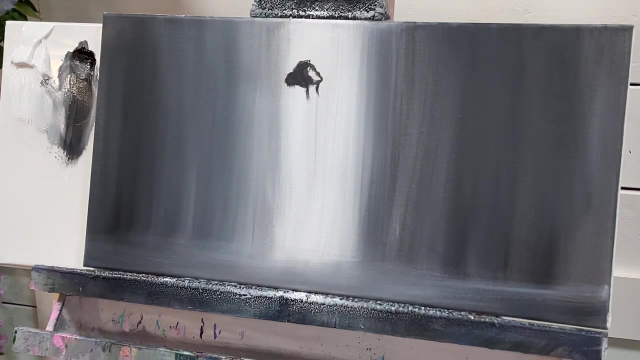 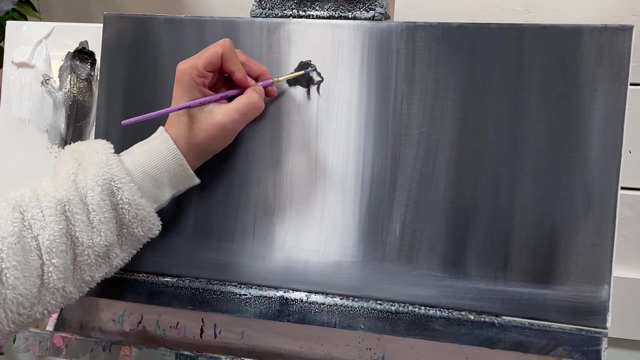 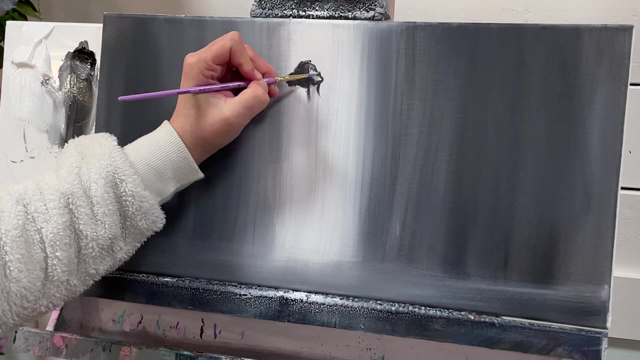 chin. we're going to come around, add some hair, a big bun, bring her neck down. I'm going to rinse my brush out and I'm going to push out the forehead a little bit while taking off a little bit of the paint. push out the nose a little bit, taking off a little bit of paint. 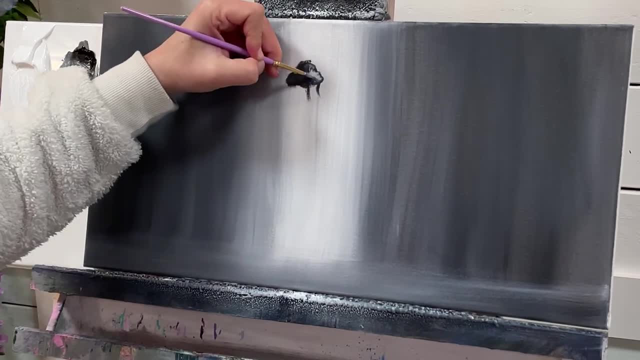 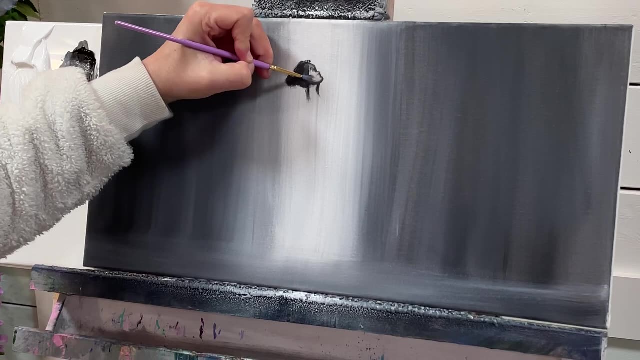 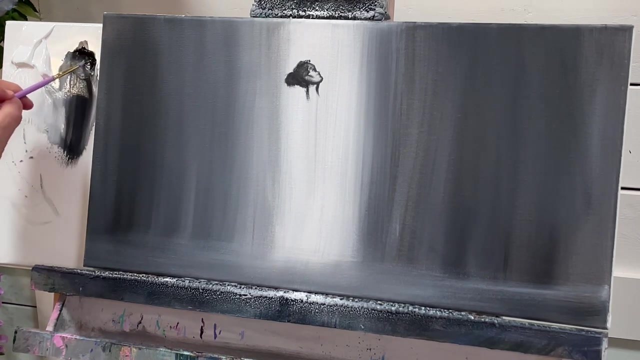 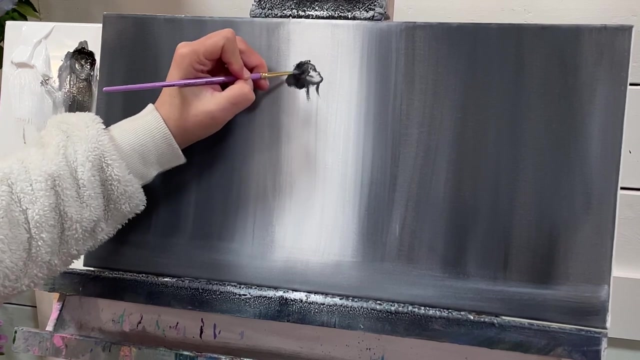 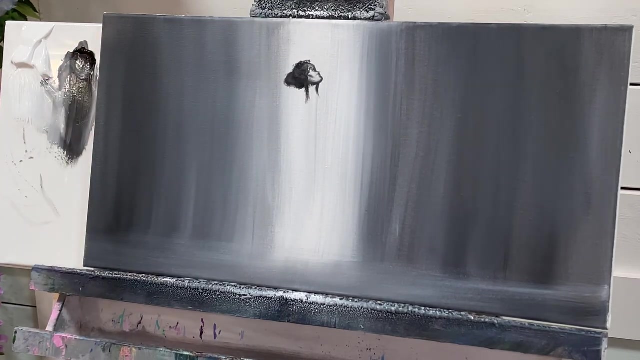 and soften the jawline and bring down the hair a little bit. I'm going to mix up a dark gray, just a little bit of white, a little bit of black. here's going to be a little lighter orange. here's going to be a little darker than this. it doesn't really matter. 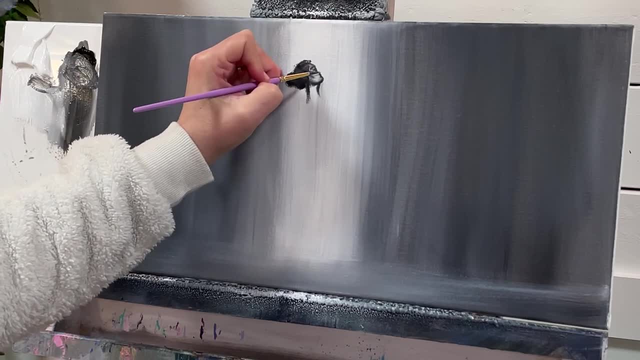 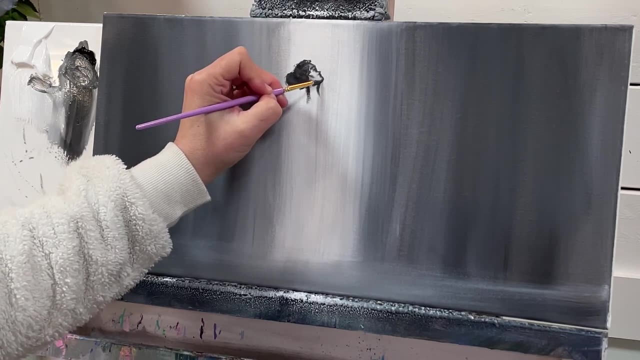 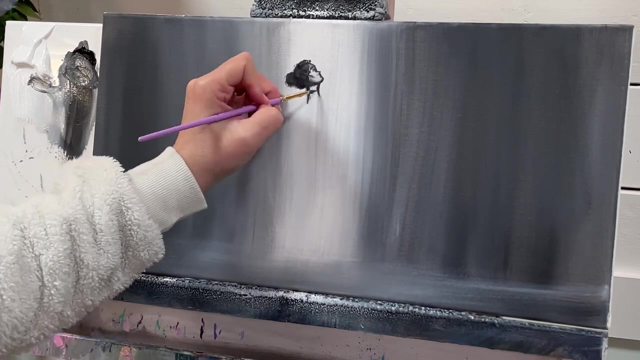 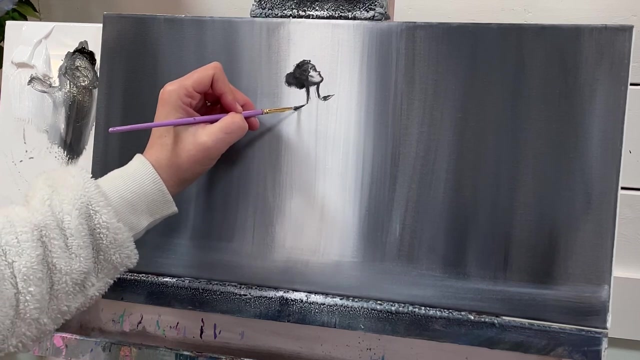 eyebrow, nose, a little bit of a mouth in there, chin, jaw, neck, and then we're going to add some shoulders here, so it's going to be on an angle. and then we're going to add some shoulders here, so it's going to be on an angle. 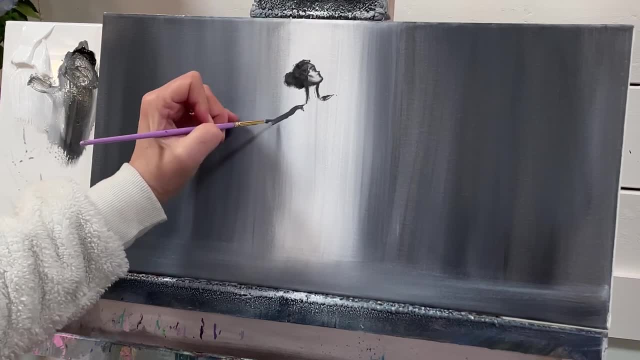 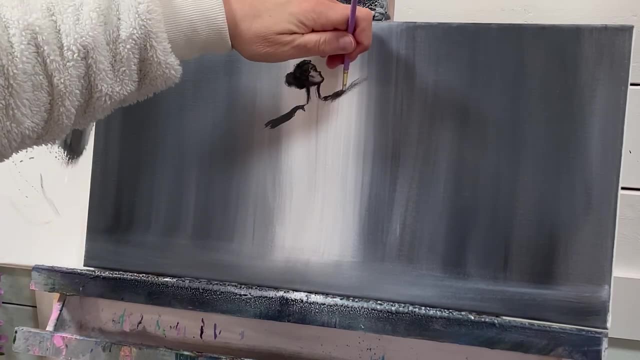 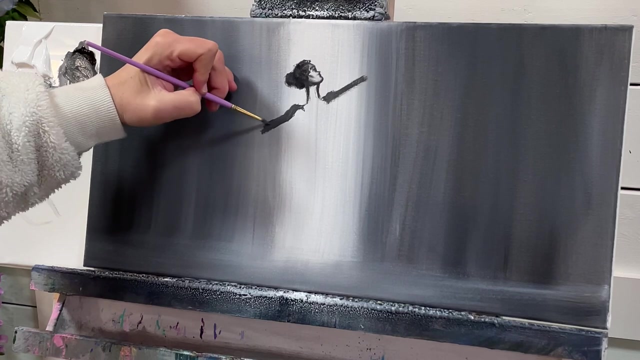 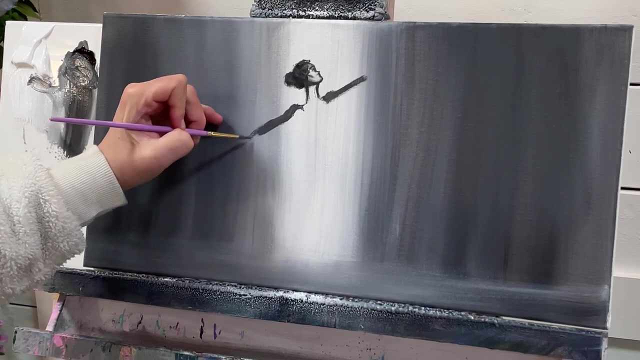 and then we're going to add some shoulders here, so it's going to be on an angle. we're going to start to pull her arms up. her elbow would be somewhere in here. then we'll add the rest of her arm wrist. her elbow would be somewhere in here, then we'll add the rest of her arm wrist. 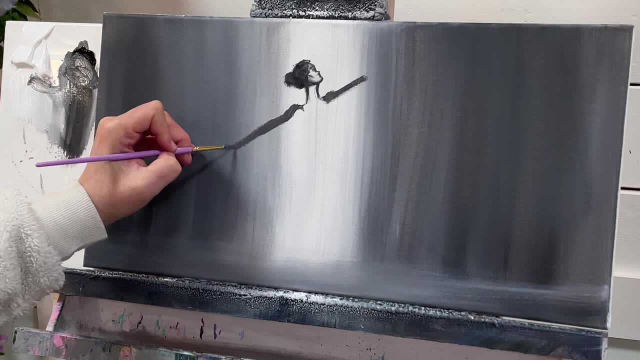 her elbow would be somewhere in here. then we'll add the rest of her arm wrist. our Nuevo is Кор tremolo. our Neveo also sounds from that color captured by a travel blog: wrist, hand and thumb. So the thumb will just come down scoop and come down here a little bit. 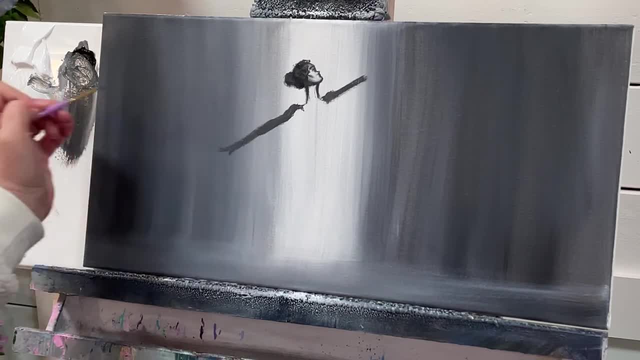 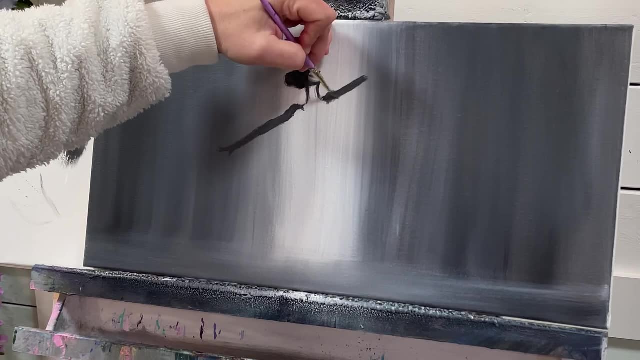 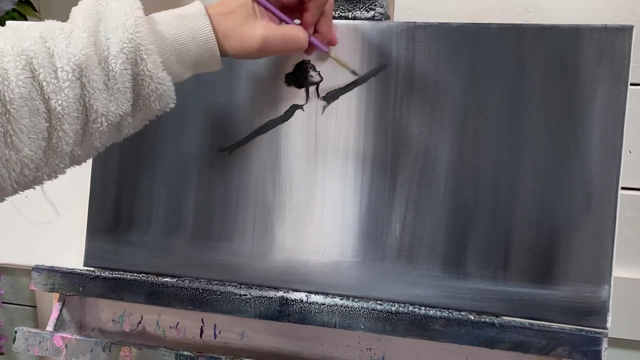 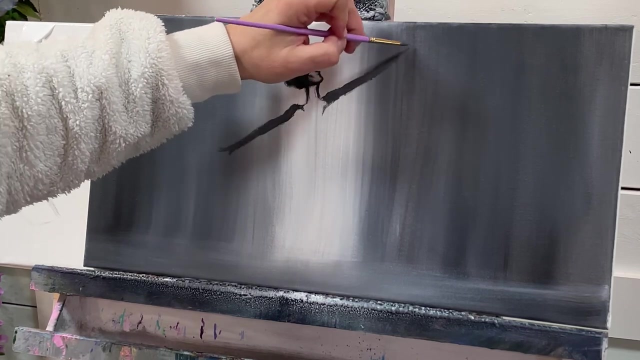 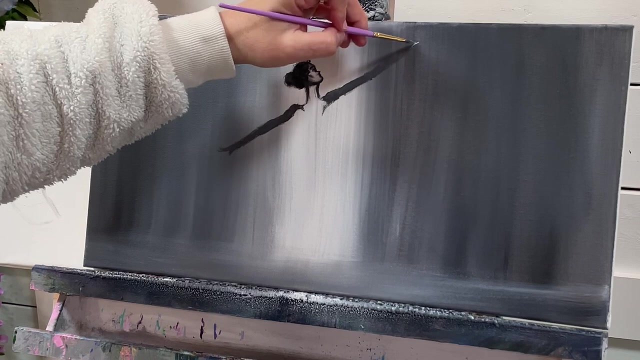 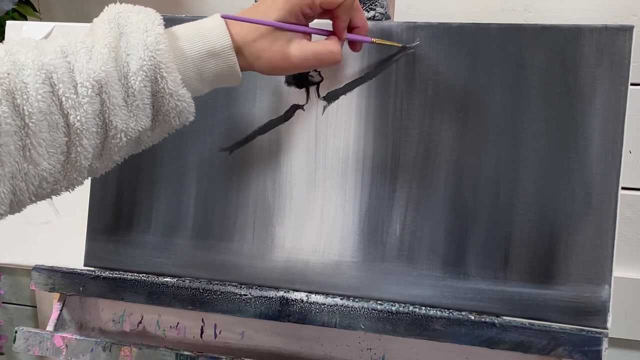 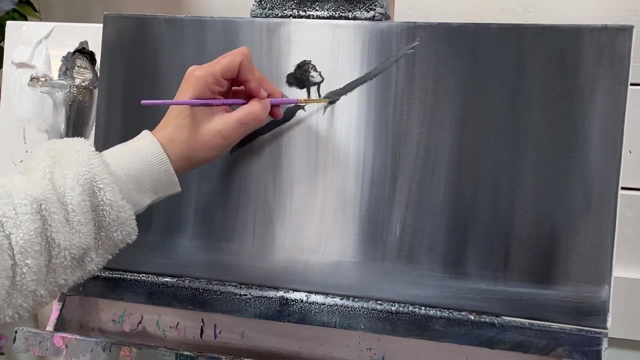 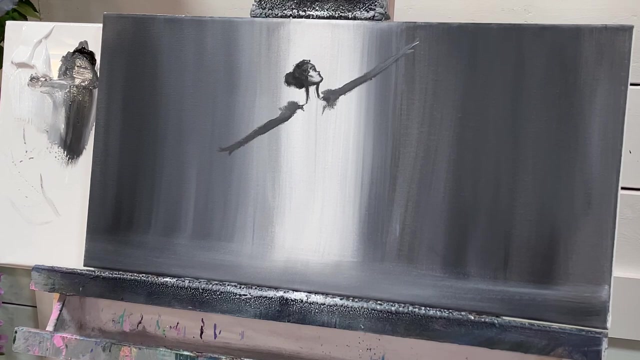 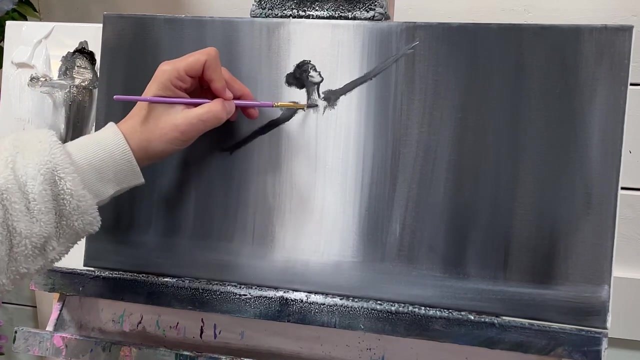 and her fingers out and then curve up. Make this a little bit wider. Her elbow will be right about here. Take a little bit of white her thumb fingers. We're gonna puff up the shoulders A bit of a shadow under her neck area here. 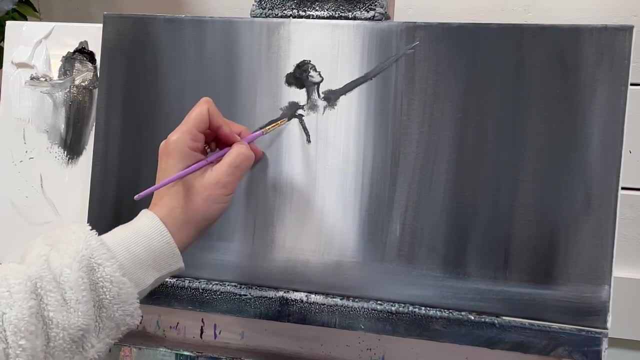 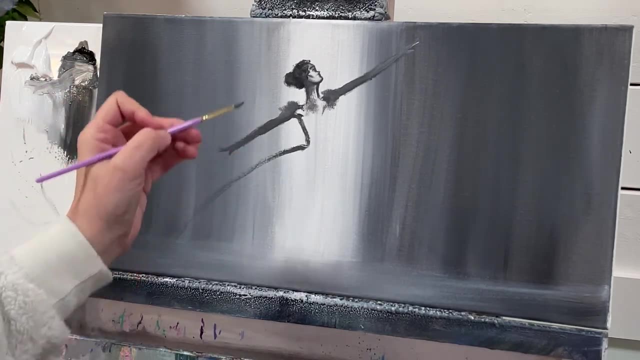 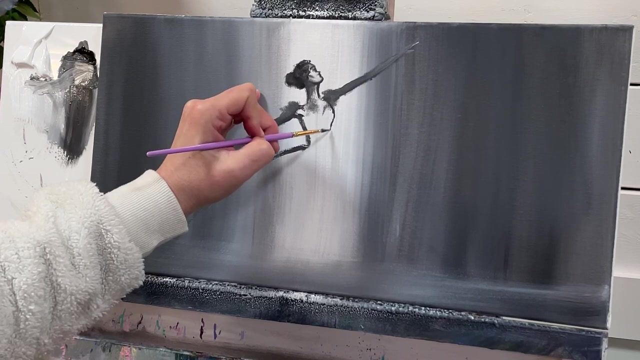 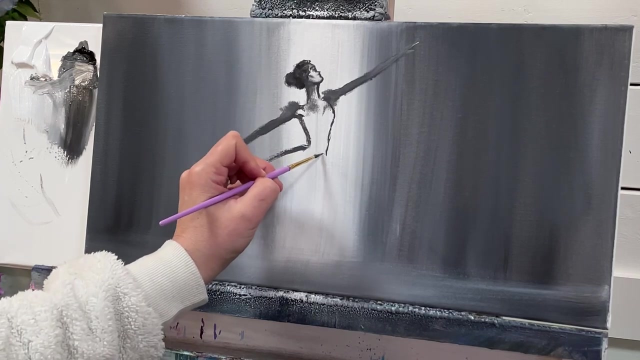 Add a curve right here on an angle, pull it in to her waist and then out for the puffy gown, Press and then in a little bit Down, a little lower, so it'll be slant like a line, a diagonal line, where it goes higher up here on the left and 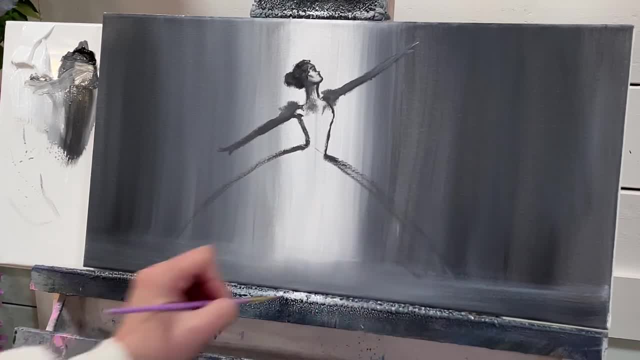 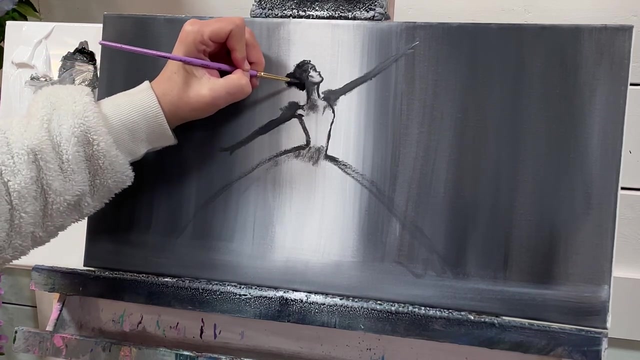 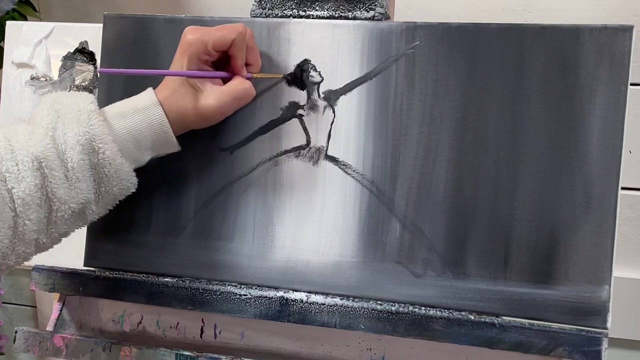 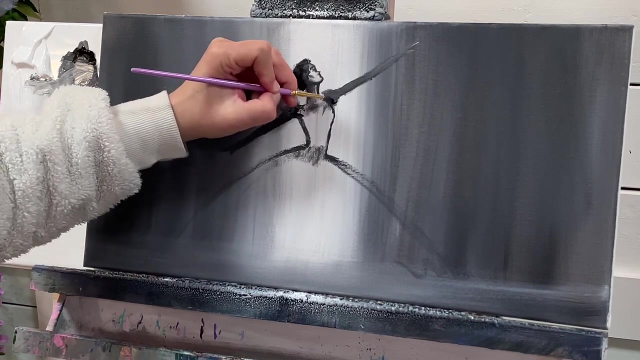 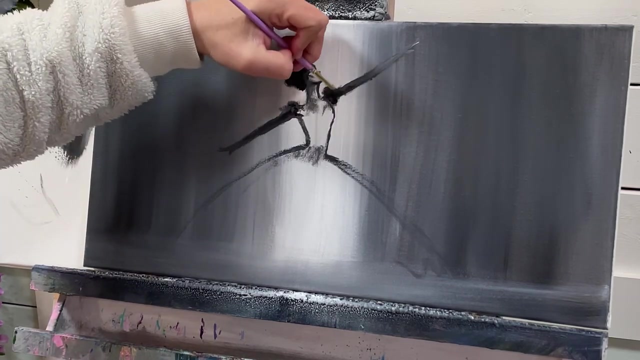 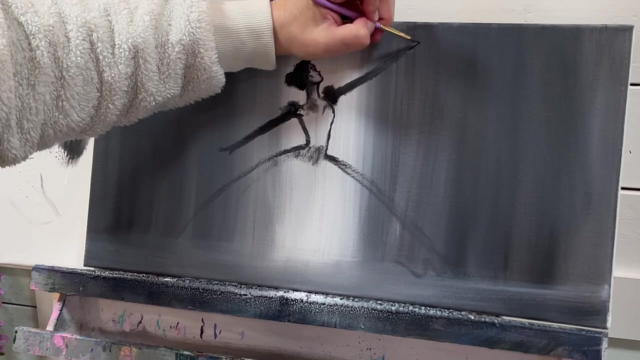 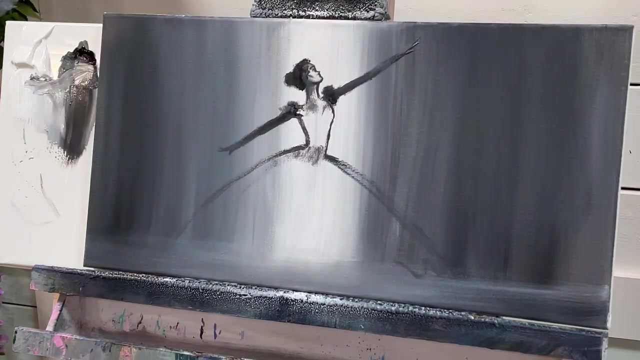 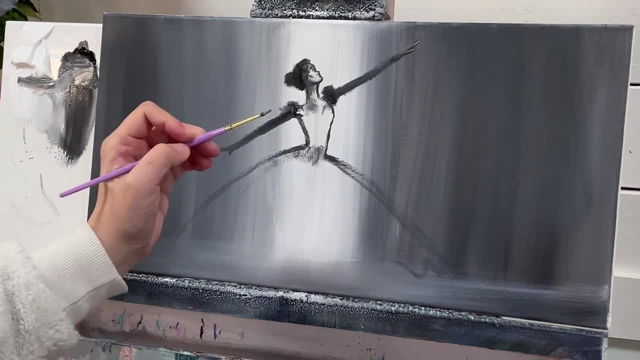 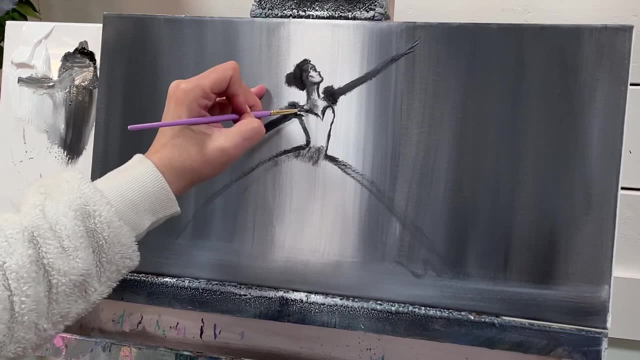 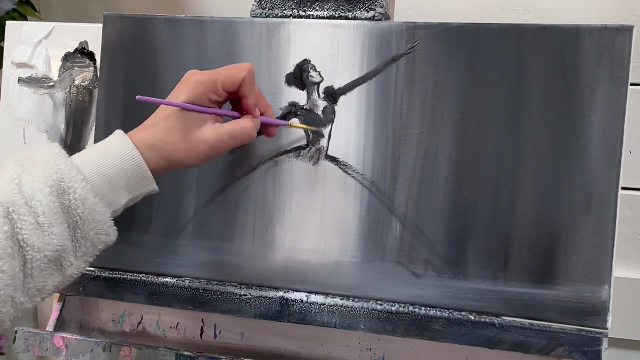 And her puffy shoulders. Okay, a little bit of dark grey. We're going to come down here and down here in the middle, And down here in the middle And down here in the middle and we're just gonna blend that paint out. 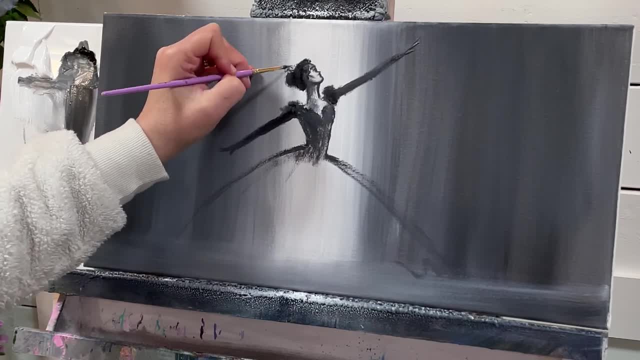 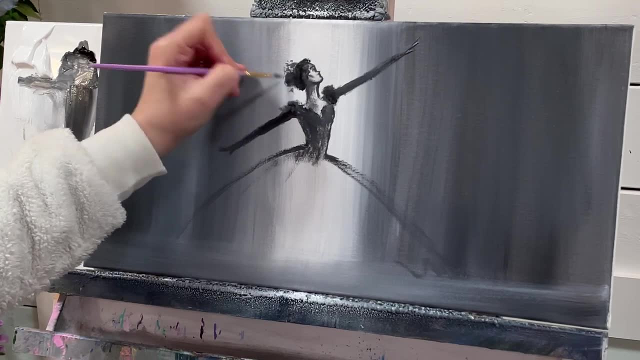 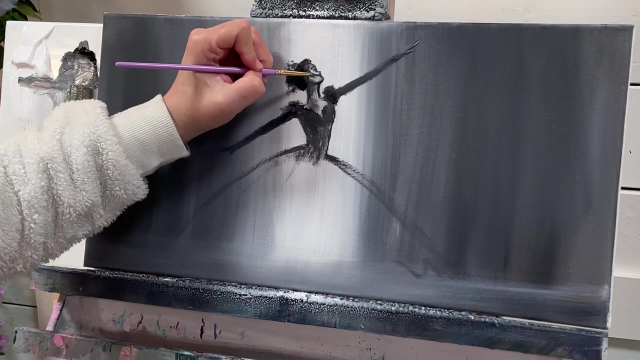 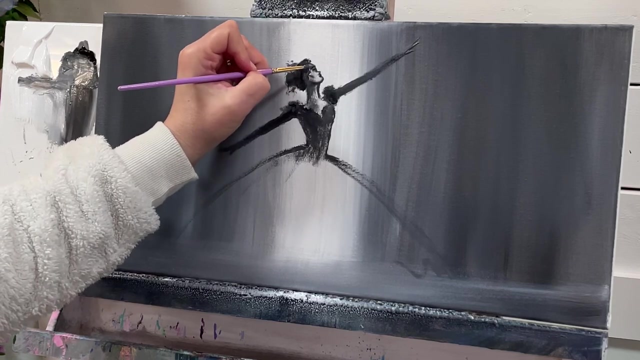 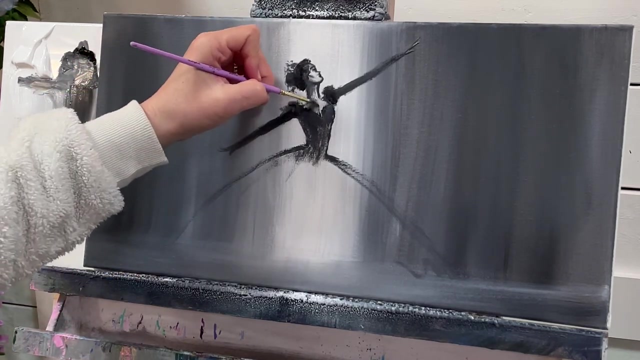 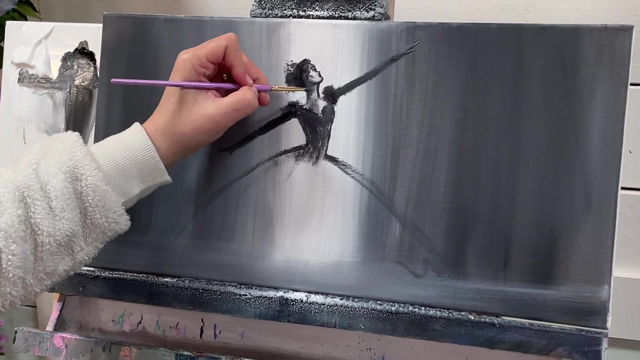 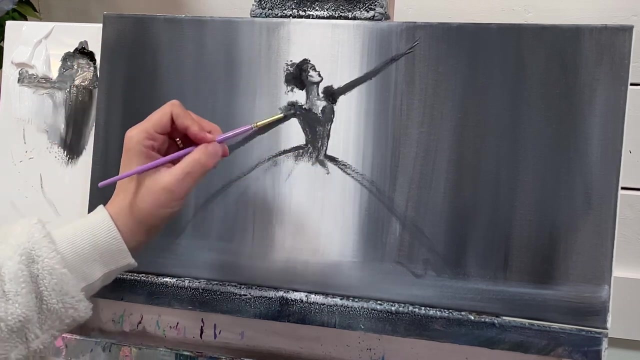 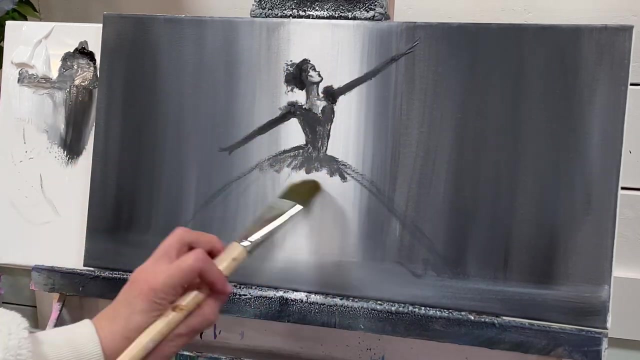 and a few little dabs here with a gray, maybe for some flowers, and take just a little bit more dark gray, black. just pull a little mouth in there, a little bit of gray, and then scoop up from the center, maybe go back over to my 30 filbert and just paint this in with dark gray. 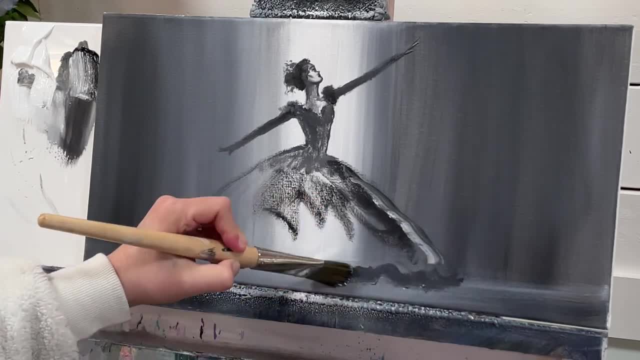 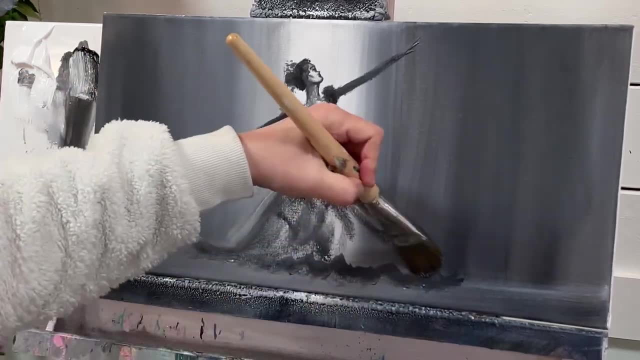 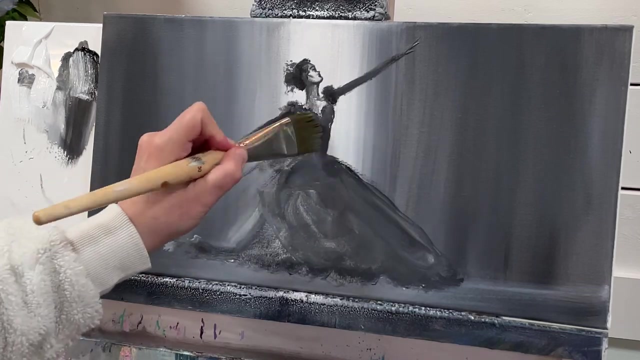 and come right down here and have it kind of spilling out over the floor, which is just want to get this kind of blocked in with this dark gray. use a little bit of water, if you need to, to help speed up the process and get it painted a little. 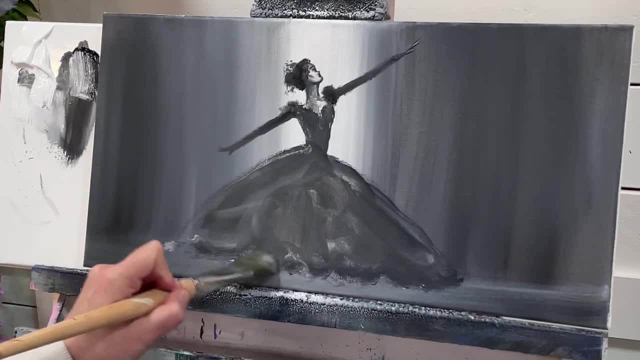 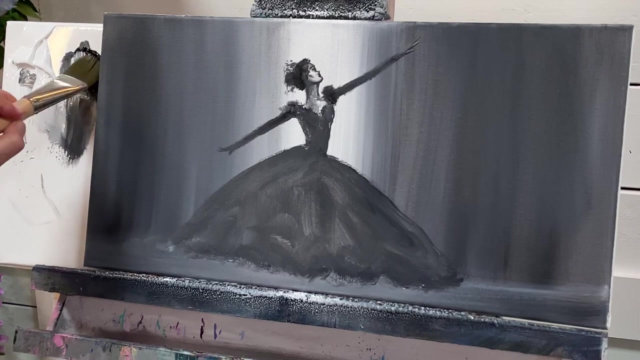 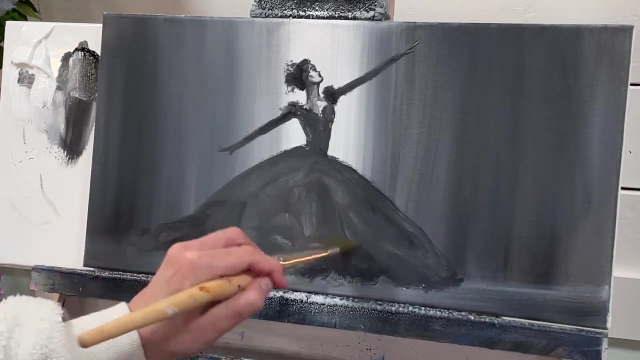 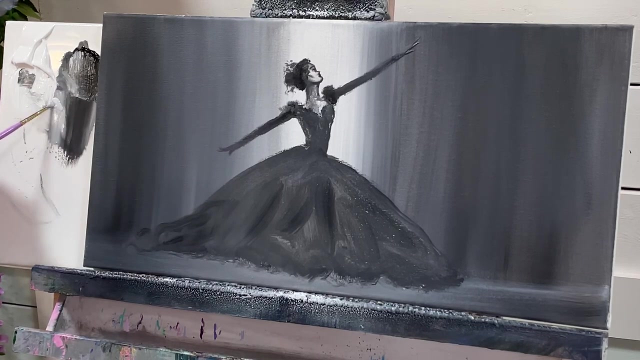 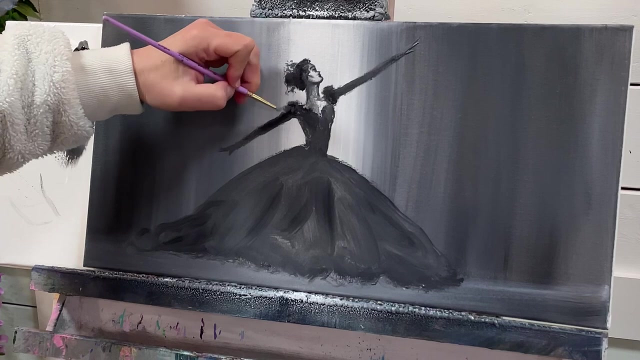 faster and then we're gonna come in and it'll be. the fun part is coming in and creating all the little flowers with q-tips. now i'm going to take a little bit of light gray, more white than black, and i'm going to add a little bit to her. 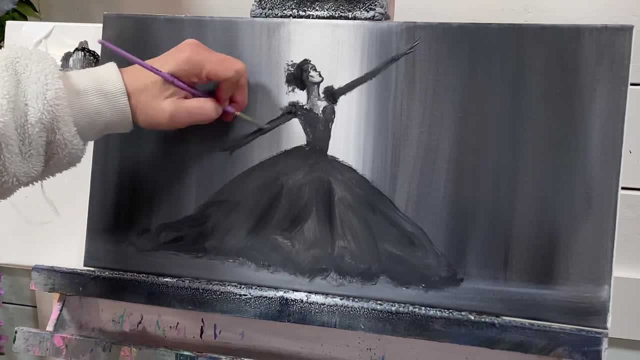 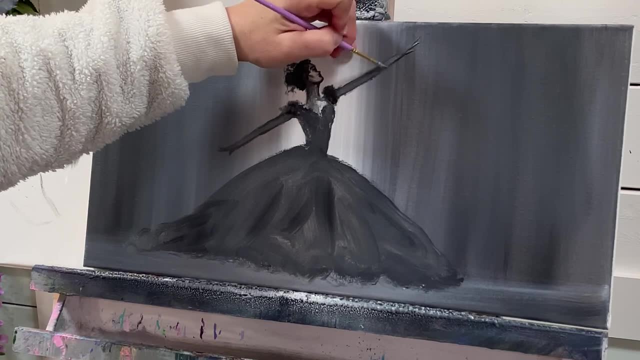 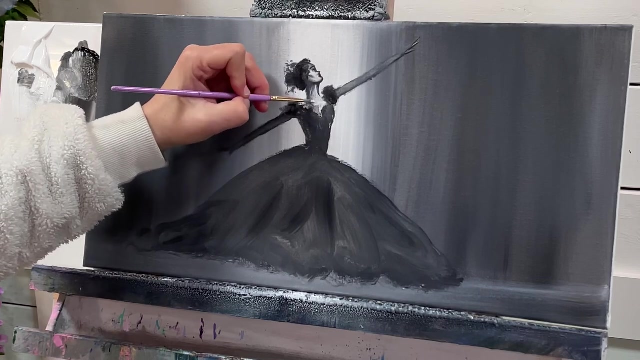 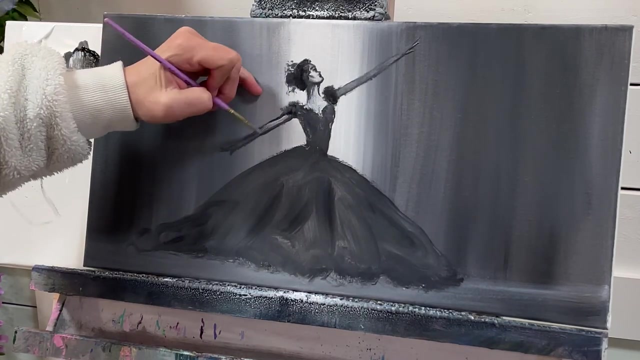 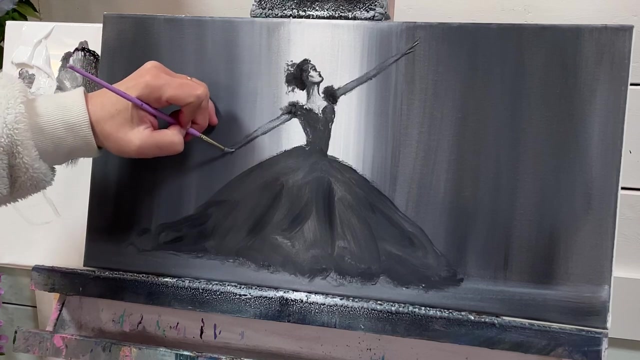 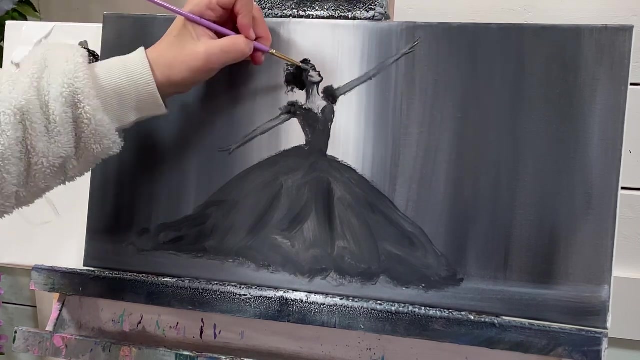 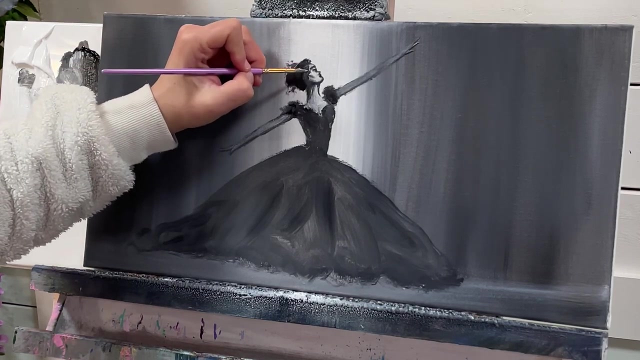 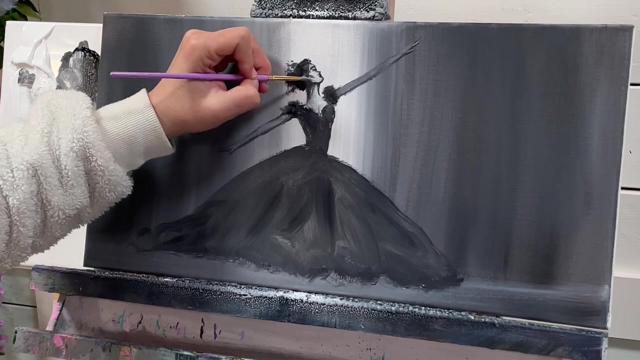 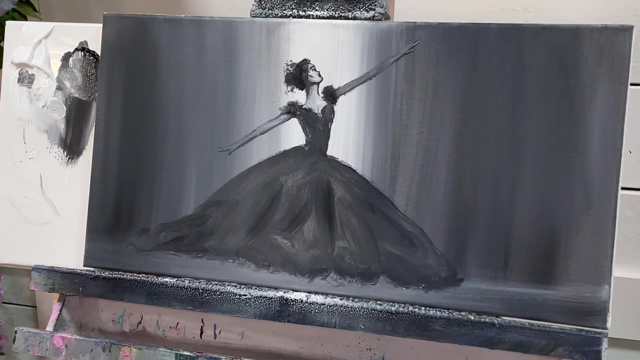 arms here so they're not completely in silhouette. take a little bit more white, soften the neck area gradually, add a little bit more just inside the outline. I'm going to add a little bit to her forehead. Okay, now I'm going to take the q-tips and I'm going to start. I've got three here you. 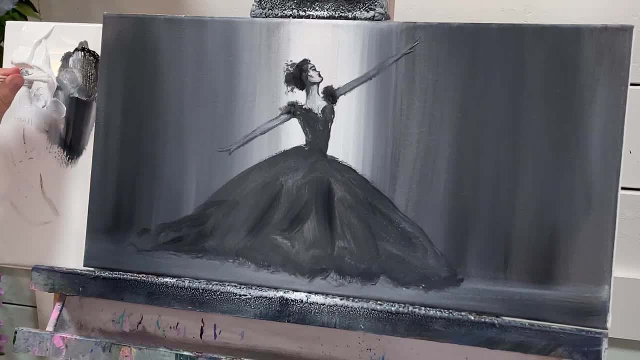 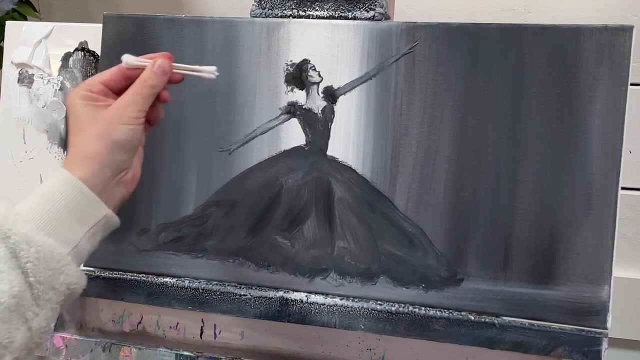 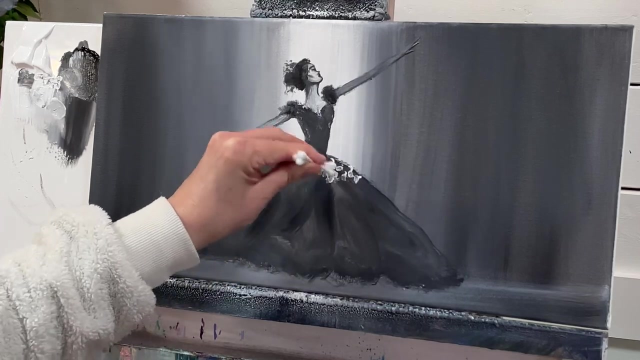 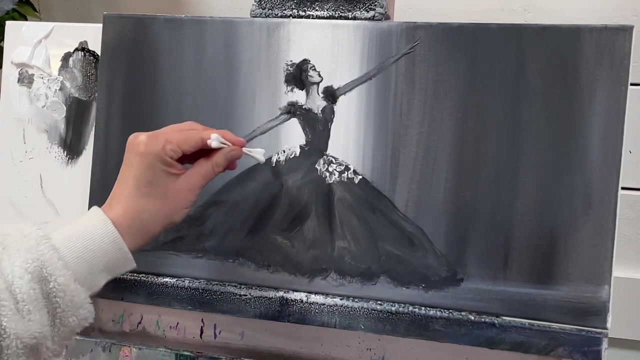 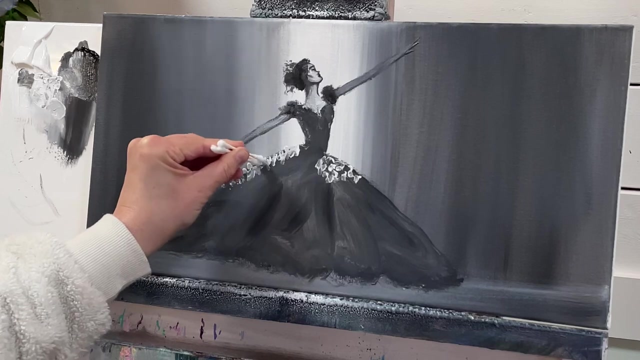 can use more if you want, and I'm going to start adding some white. Just dab it into the white, Okay, And just tap away and it's going to look like little flowers. Now I'm adding these outside of the outline so they look 3D and like the petals are sticking. 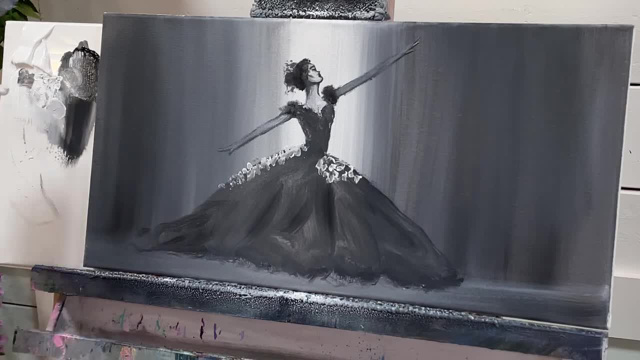 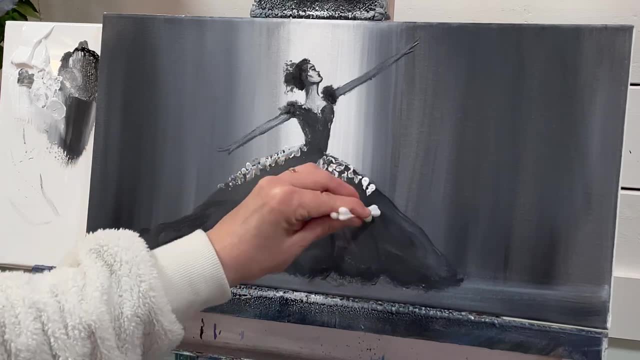 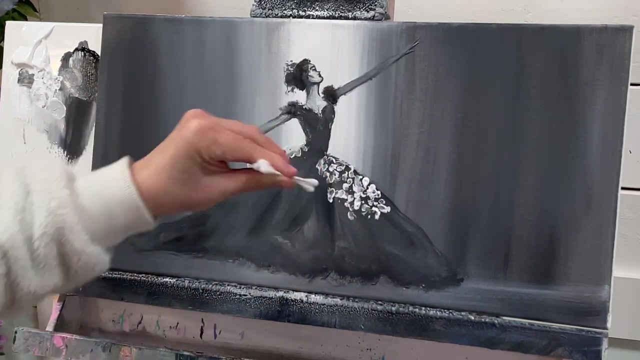 out. If you want to do this, one q-tip at a time, you can. You can use more than this if you want. I like to push and tap and then turn each time, so they're in a different direction and it looks a little. 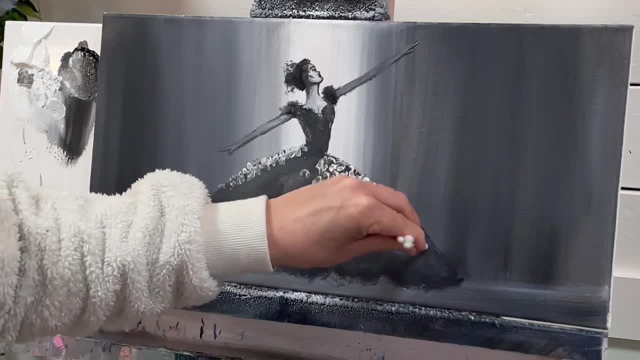 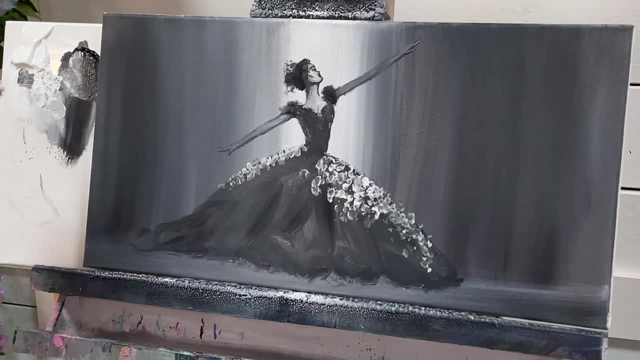 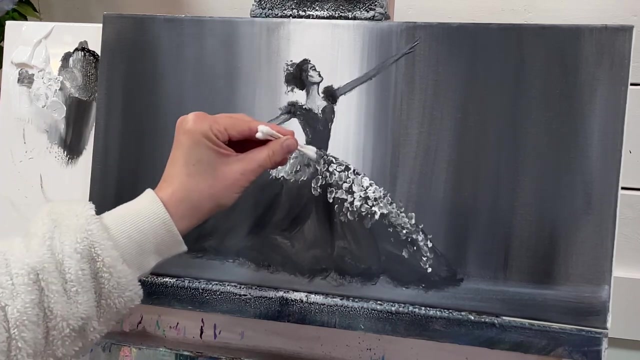 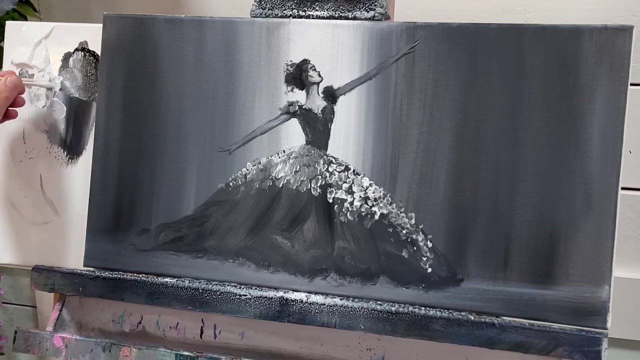 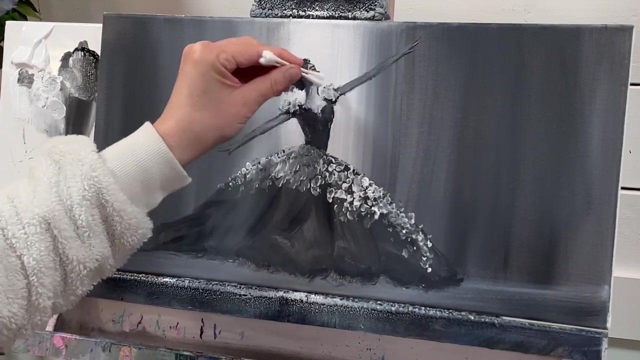 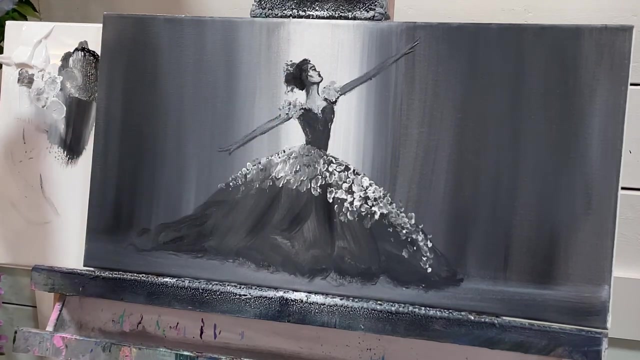 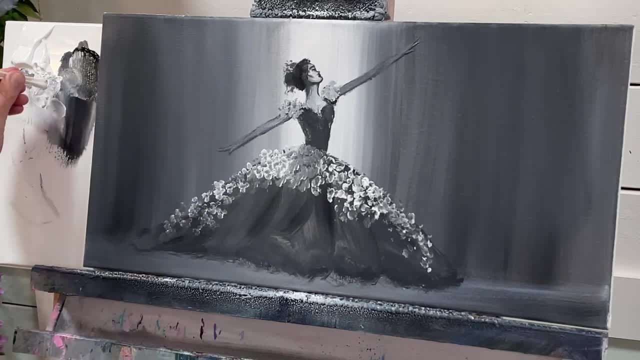 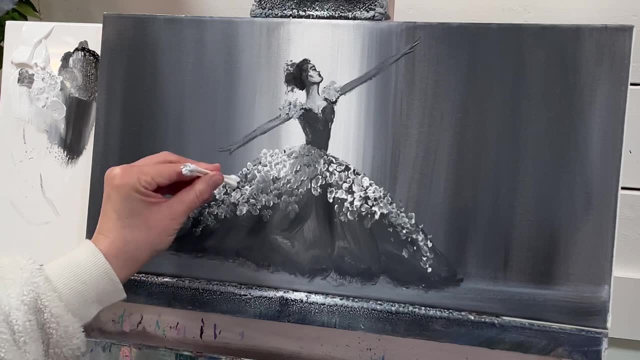 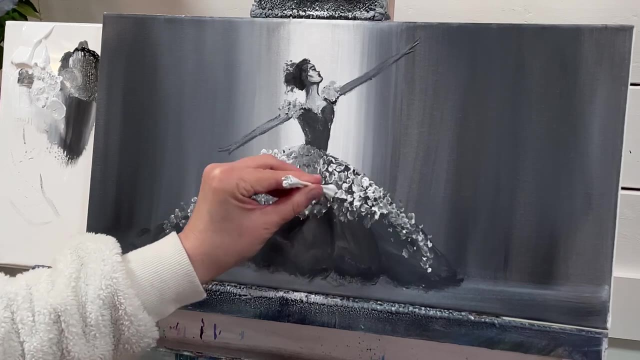 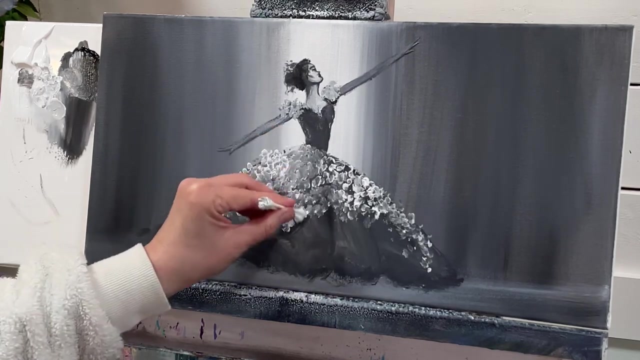 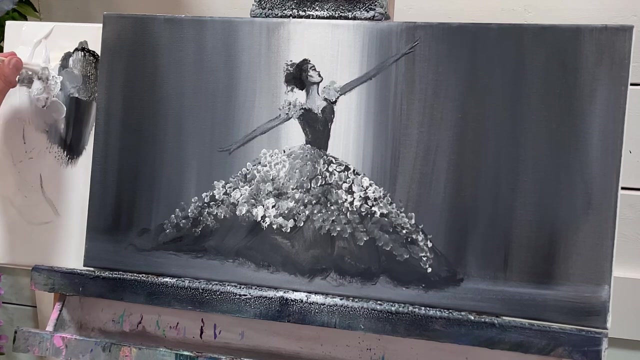 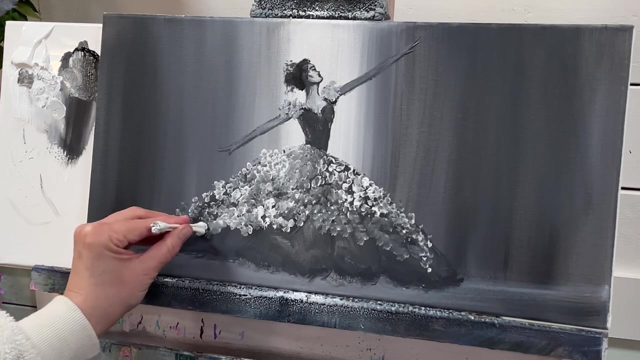 Okay, Okay, Okay. I'm going to add lots of little ones here on the biggest part of the dress and then down here I'm going to show you a different technique with the q-tips to make it look like bigger flowers. So I'm going to start making them a little bit bigger and I'm going to push and twist. 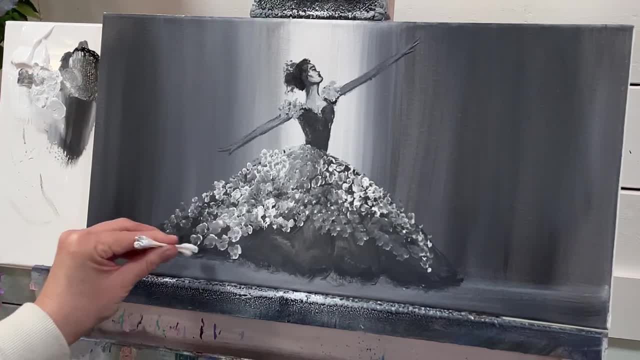 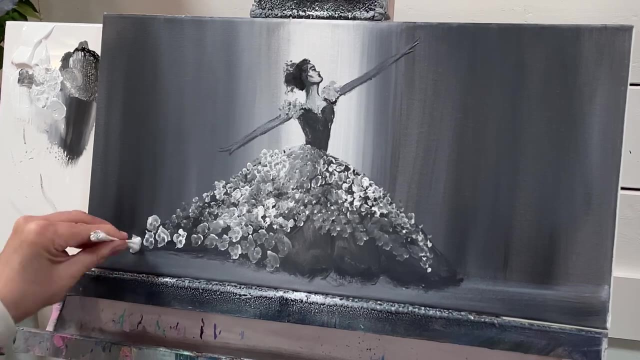 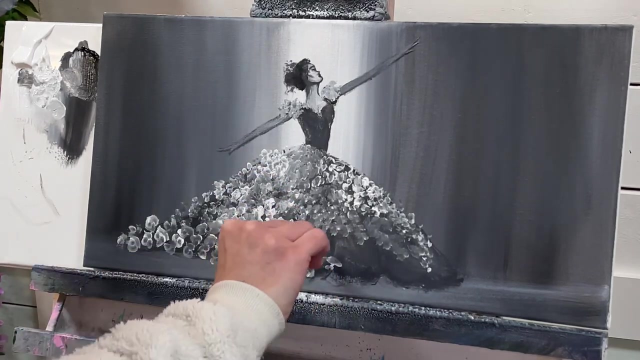 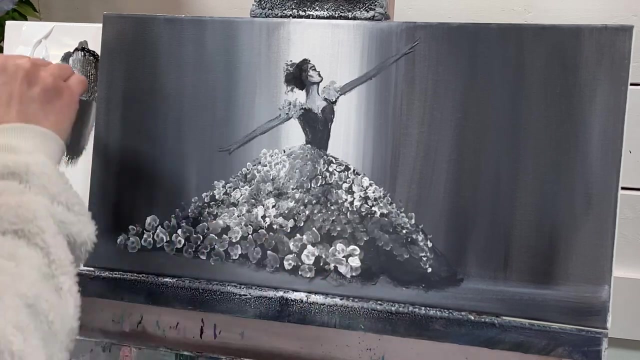 load my the ends up, push and twist. Okay, So I'm going to go ahead and do that, and then I'm going to go ahead and do that again. Okay, So I'm going to go ahead and do that, and then I'm going to go ahead and do that again. 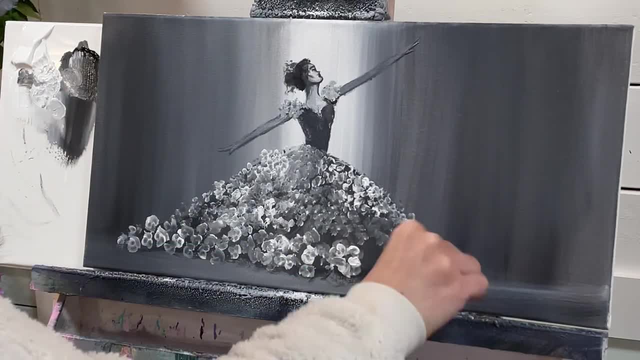 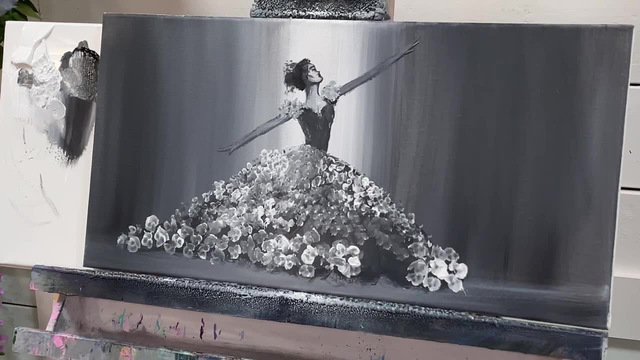 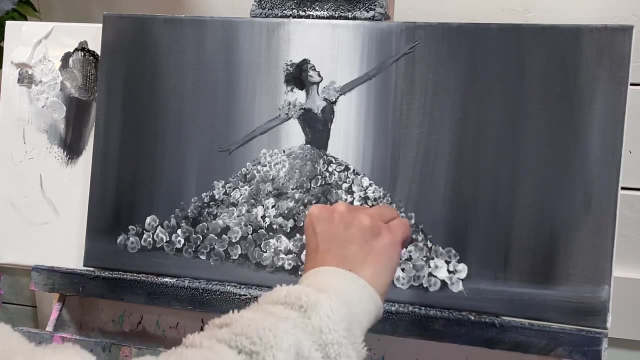 Now I like doing this on a wet underpainting, because then it picks up a little bit of the dark gray and you get different shades. But look at how elegant this is and we're using q-tips, so you really don't have to have. 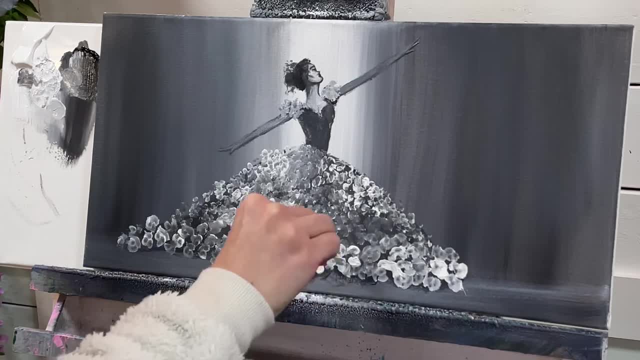 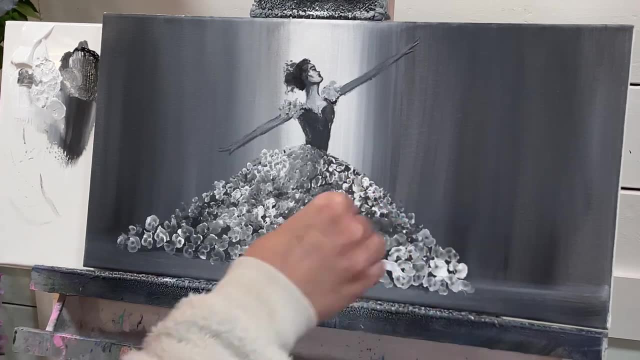 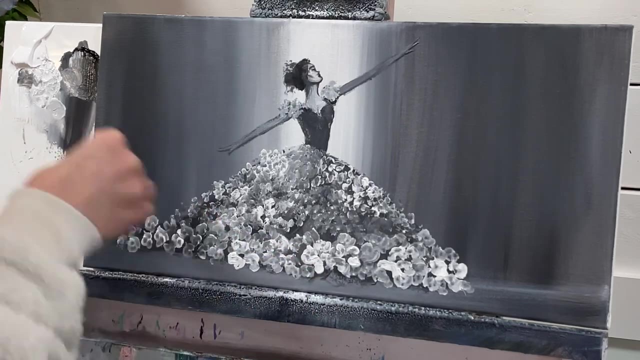 fancy brushes. Having good brushes is nice for certain things, but think outside of the box and don't always think that you need them to create something wonderful. So again, we're concentrating on bigger flowers at the bottom and then smaller ones At the top. 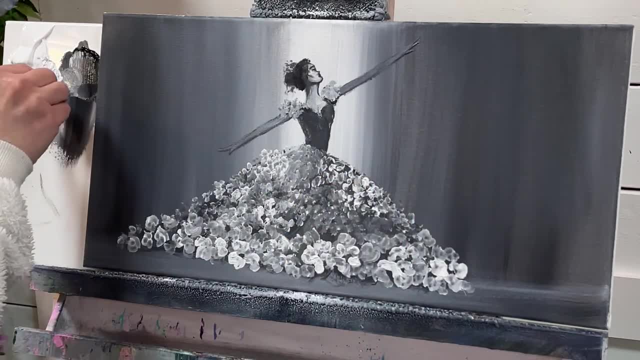 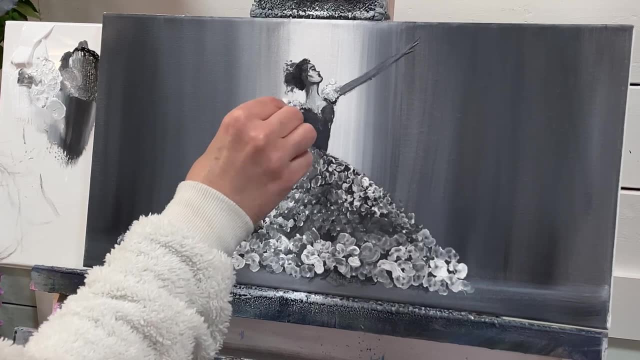 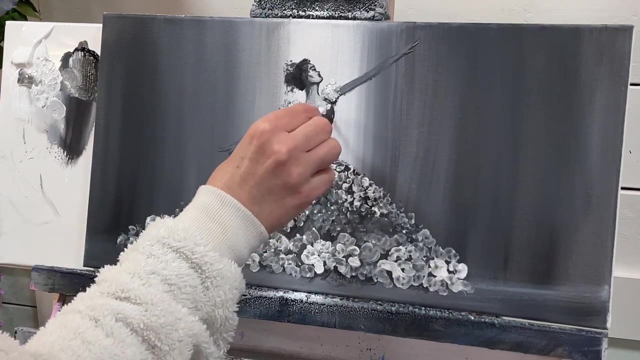 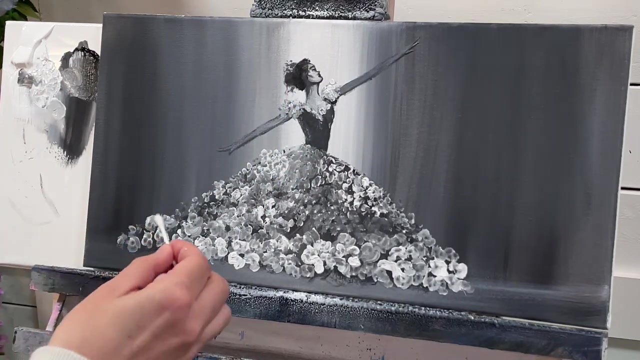 So I'm going to take a clean q-tip and I'm going to dip into the white and I'm going to add little dabs. I'm going to dab along her, the top of her dress, Okay. So that's that Okay. 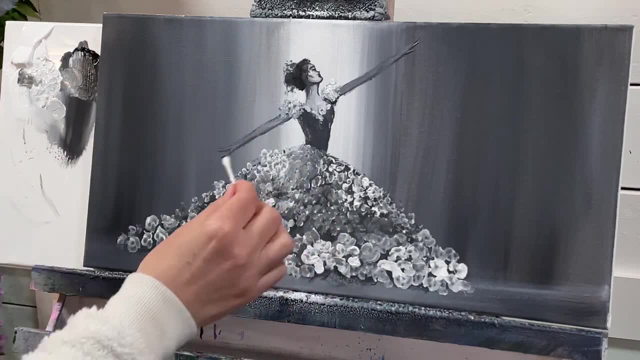 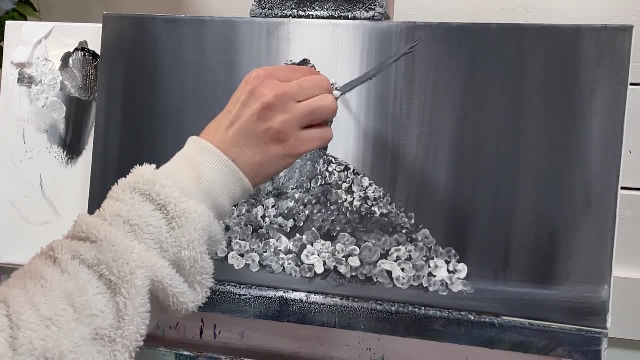 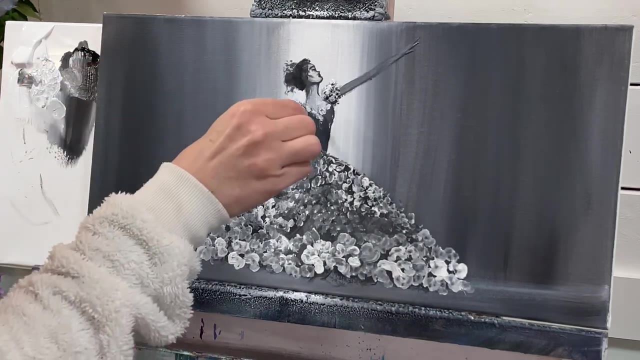 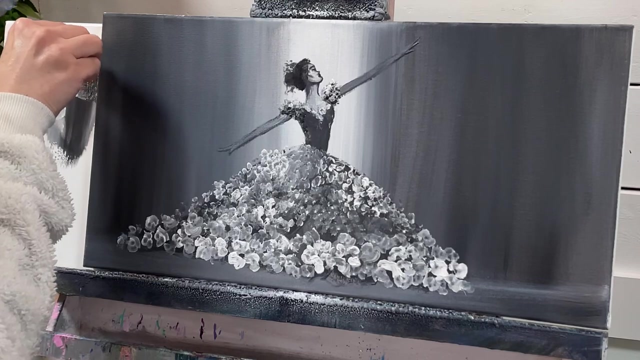 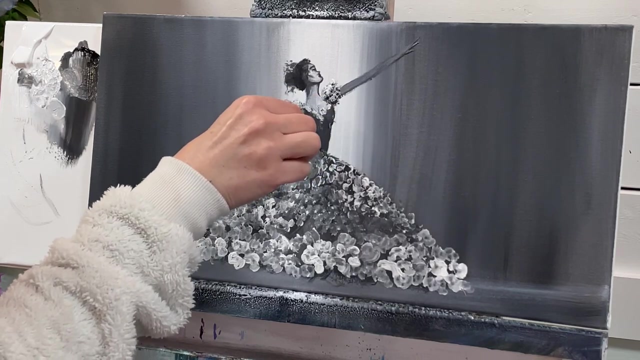 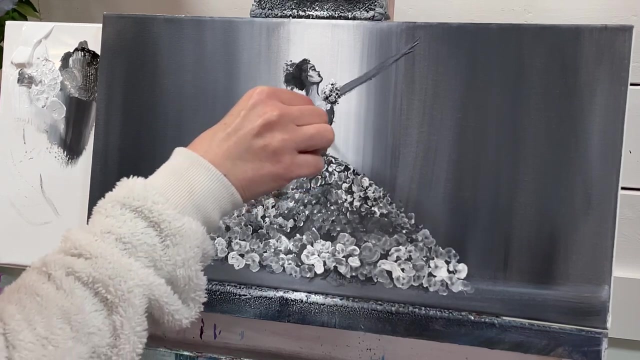 I'm going to take a little bit of black too and I'm going to add it in here to break up a little bit of all the light gray and white. so we still have some contrast and some shadows, a little bit of black spreading, a little bit of shading right in here. 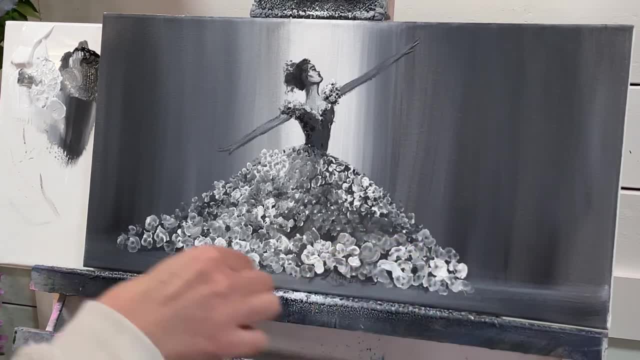 I'm going to add a little bit down here, and I'm going to add a little bit down here. I'm going to add a little bit down here. I'm going to add a little bit down here. wherever you envision a big flower, you can make them look like really stand. 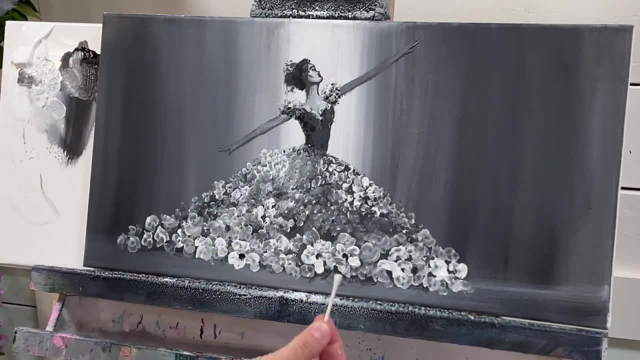 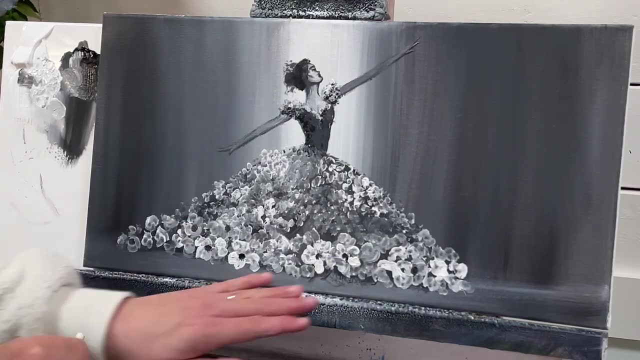 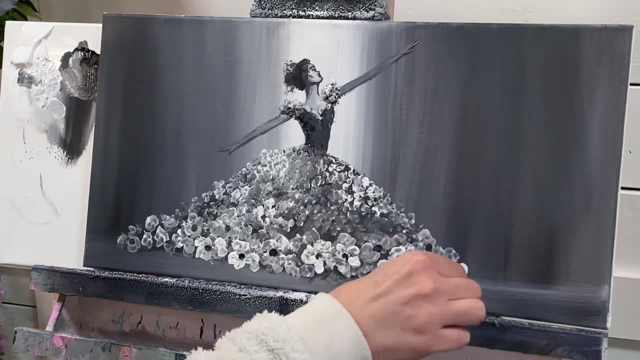 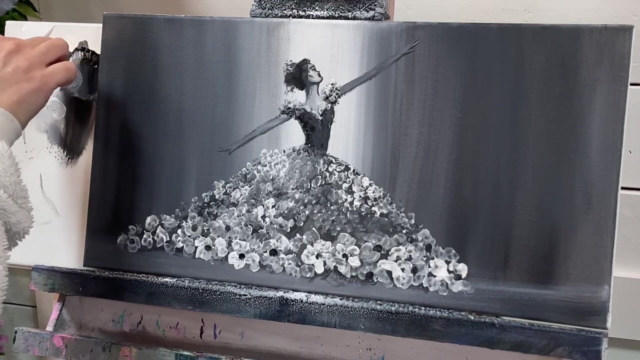 out to be bigger flowers now by adding a little dab of black inside. just these ones down here, though, just these ones down here, though you're going to take a little bit of black inside and we're going to add more here, more weight, and I'm going to come. 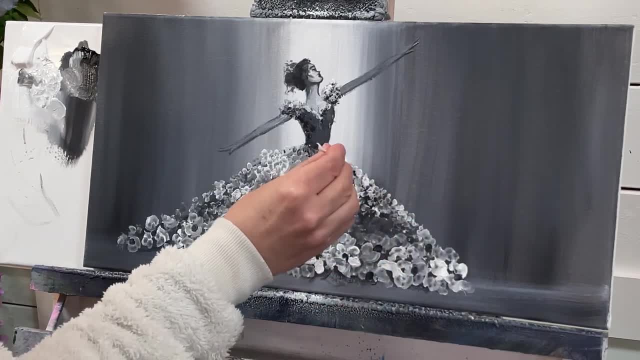 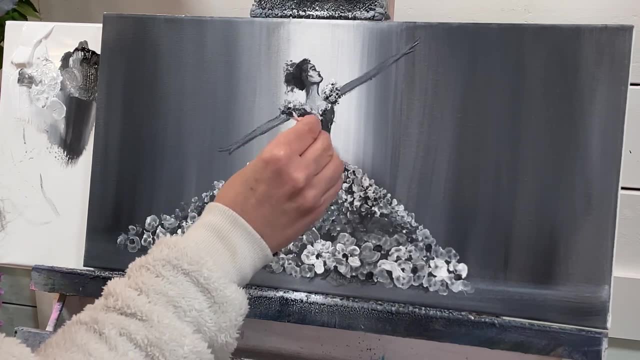 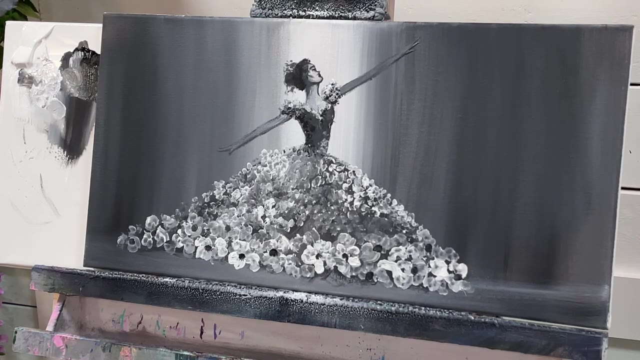 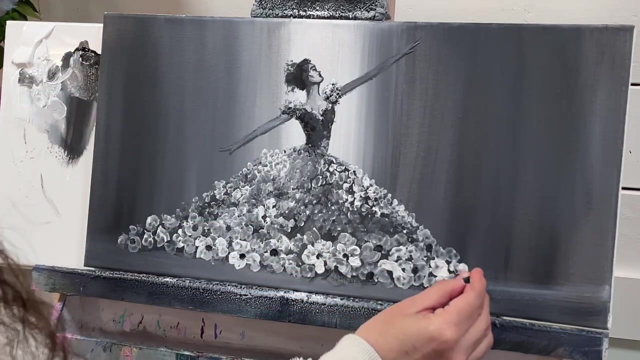 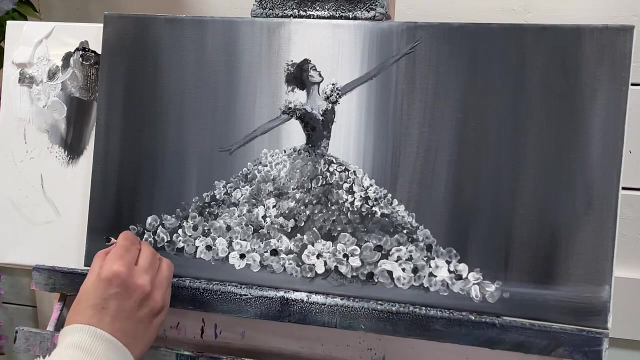 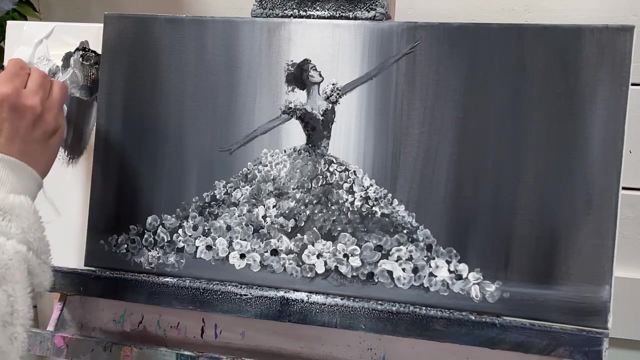 along the outline of the dress in the front. take a little bit more black and white to make some gray. I'm going to start to just roll and twist my brush around and let's get all those q-tips again. well, all three of them, and let's start. 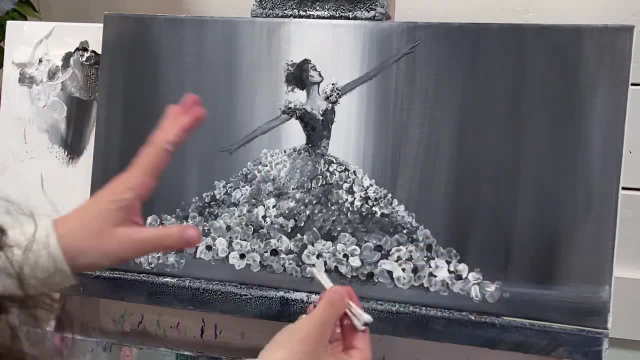 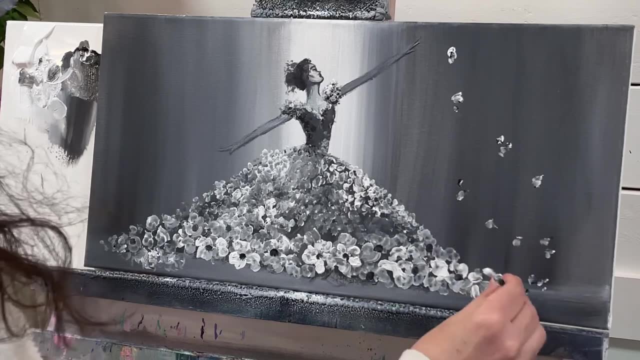 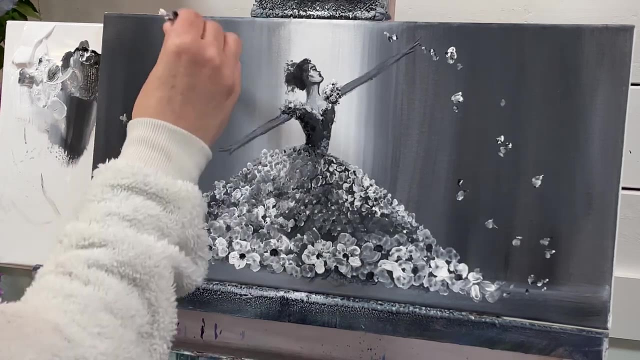 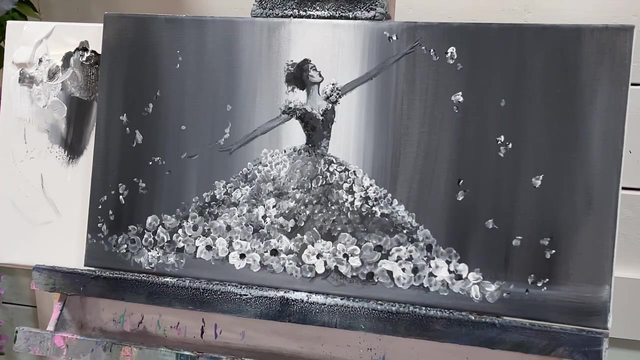 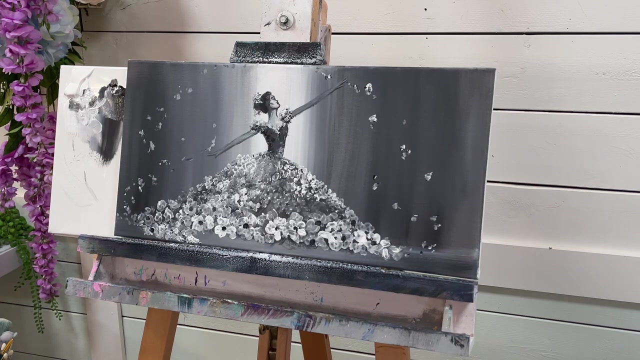 to get a little loose and free and just have petals kind of falling around. I'm going to add a little bit in here, little dab of black. I'm having so much fun with this. I can't wait for you guys to try this one and this paintings all done. I loved this. hope you guys enjoyed this one too. let. 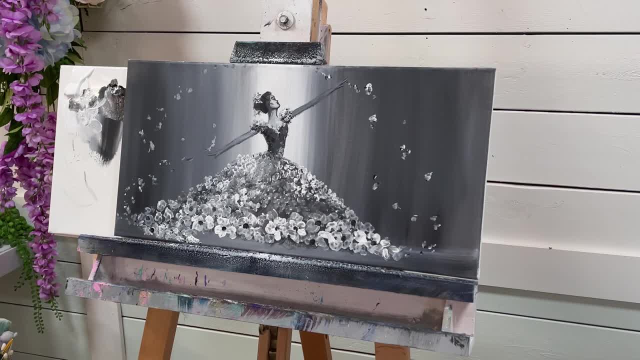 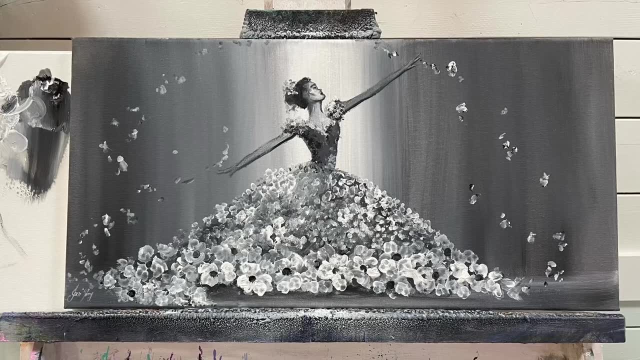 me know what you think in the comments below. have fun painting yours. don't forget to subscribe to my channel for more, and I'll see you very soon in my next video. you.